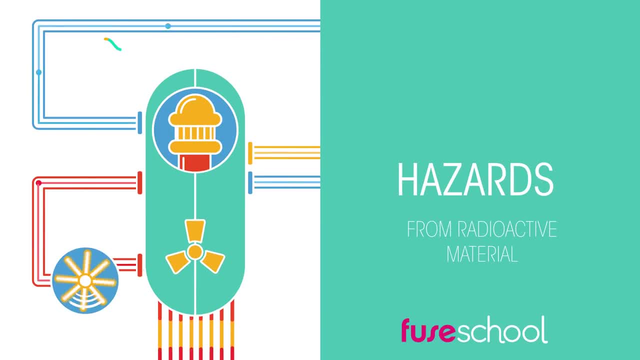 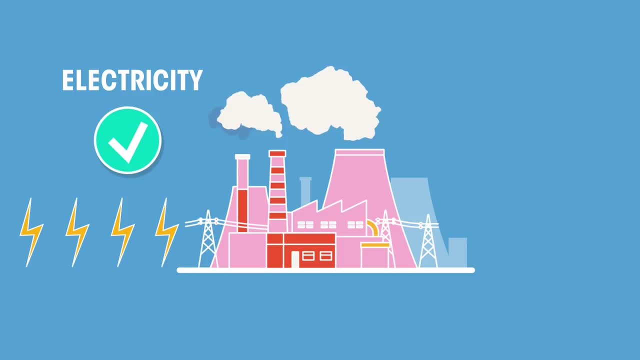 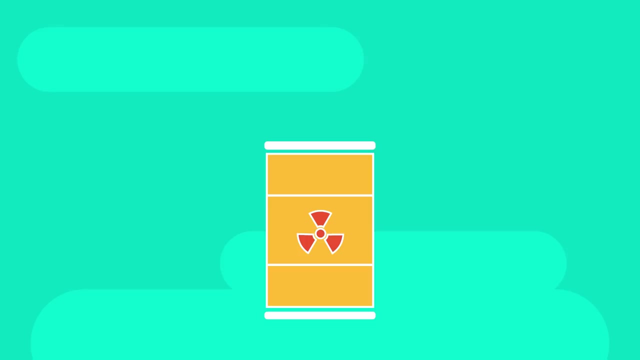 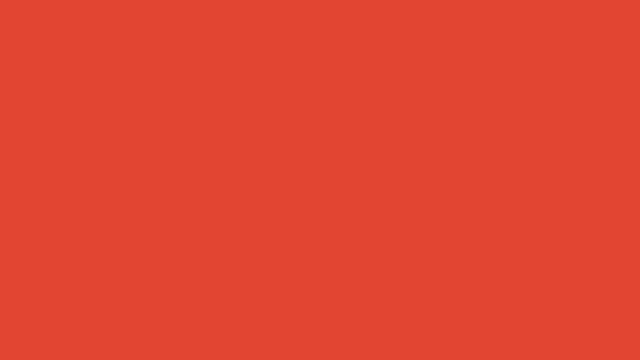 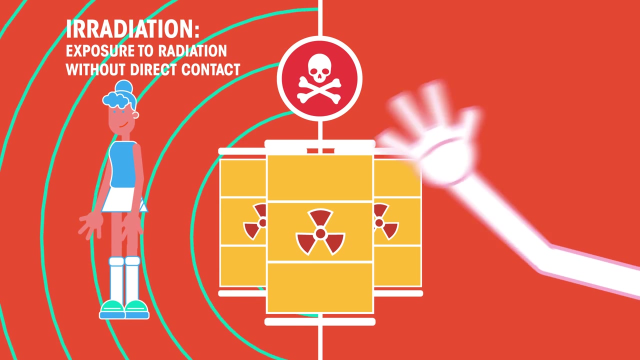 Nuclear power stations produce electricity, which, of course, is extremely useful. However, they also make radioactive waste. Radioactive waste can come from a range of activities, including generating electricity from nuclear power stations, treating medical illnesses and conducting research. Did you know that radioactive waste can be harmful to us, either by irradiation or contamination? 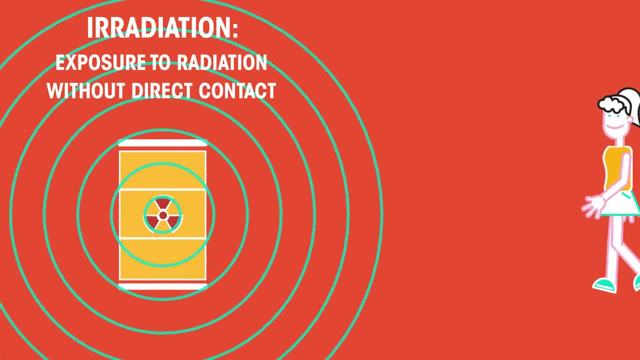 We're going to look at these two in this video. Irradiation is when a person or object is exposed to radiation without coming into direct contact with the radioactive source. The person doesn't make direct contact with the radioactive barrel, but since irradiation can happen at a distance, the person is still at risk. The 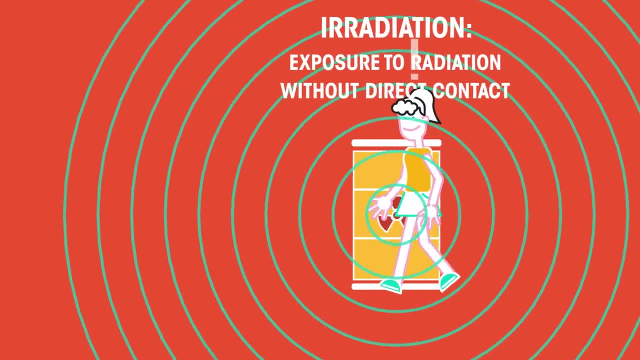 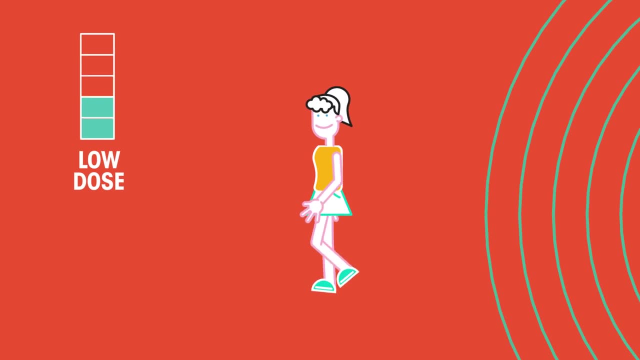 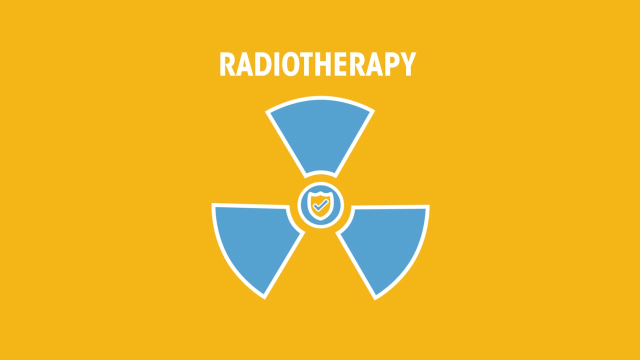 damage to the person only happens when the person is exposed to radiation. Irradiation is in the area of the radioactive waste. Therefore, the person is only exposed to the radiation for a short time and so receives a low dose of radiation. Irradiation can sometimes be useful, particularly during cancer treatment. People are irradiated. 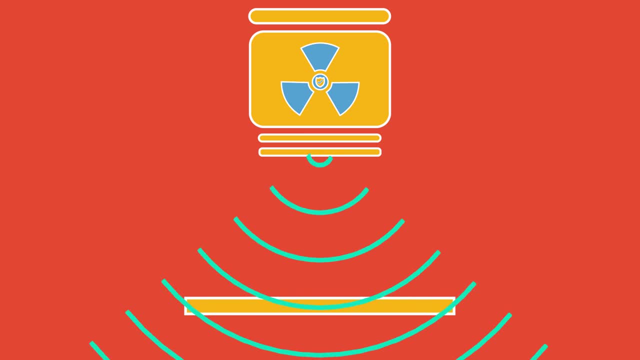 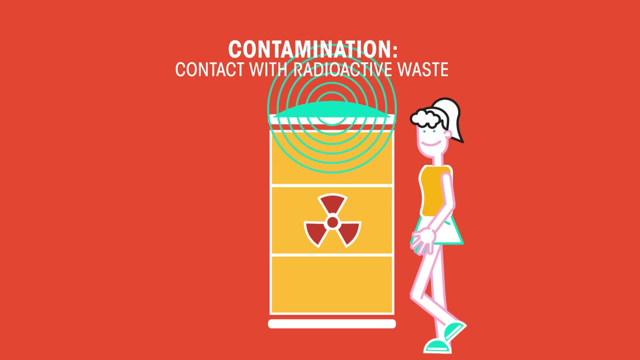 in an attempt to remove cancerous cells from their body. Irradiation is also used to sterilise surgical equipment or to remove bacteria from fruit in supermarkets. The objects don't become radioactive themselves and so are safe for use or consumption. Contamination is when a person actually comes into contact with the radioactive wastes. 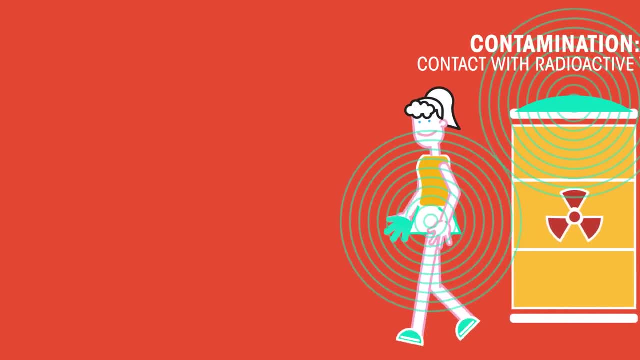 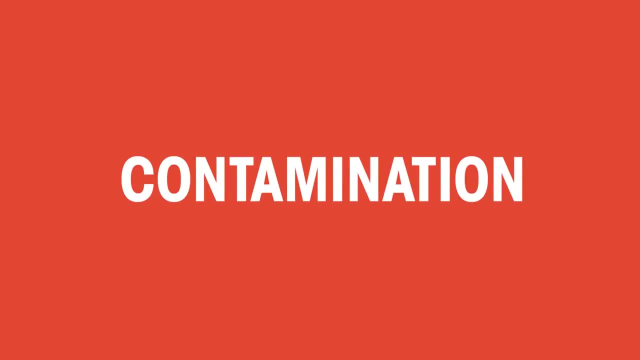 The person takes the radioactive source away with them and so are exposed for a longer period of time and consequently have a higher dose, which can lead to more damage. Contamination can happen in a variety of ways, from picking up a source to breathing it. 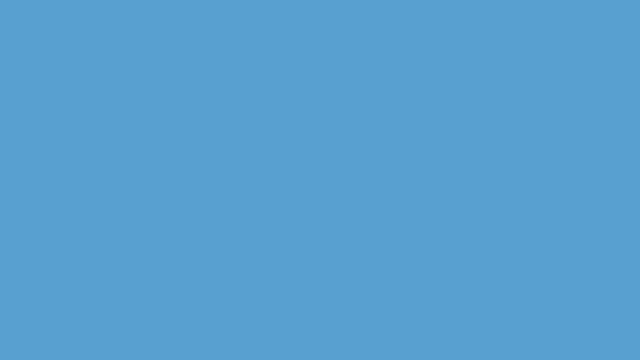 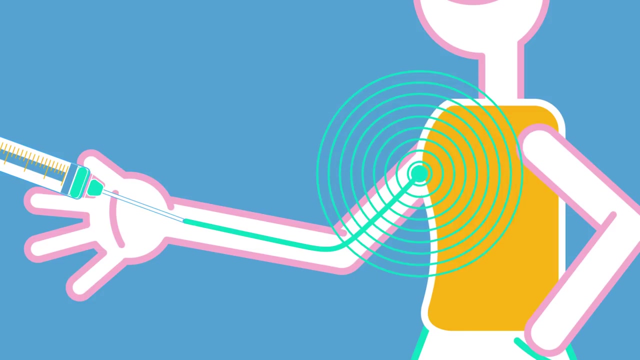 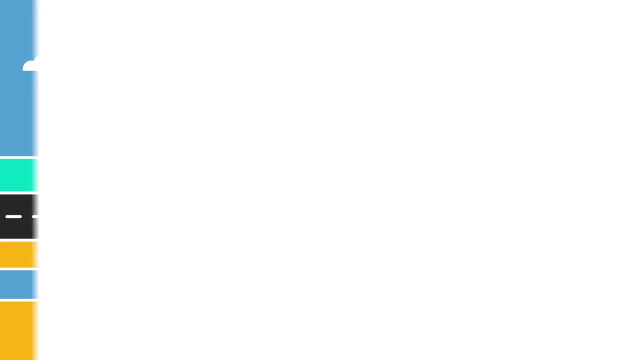 in and to ingesting it. Contamination is used in medicine by injecting radioactive tracers into the body to see possible blockages. Radioactive tracers are also used to find leaks in water pipes. Radioactive waste can remain hazardous for a very short or a very long period of time. 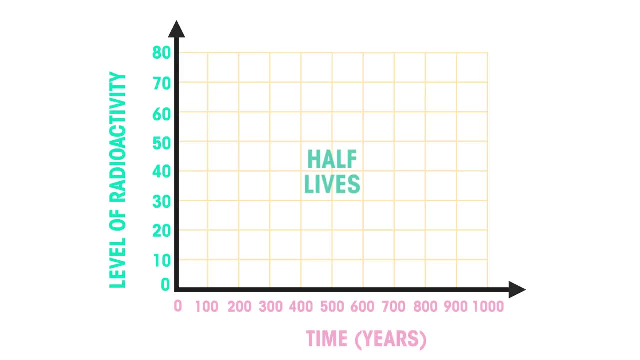 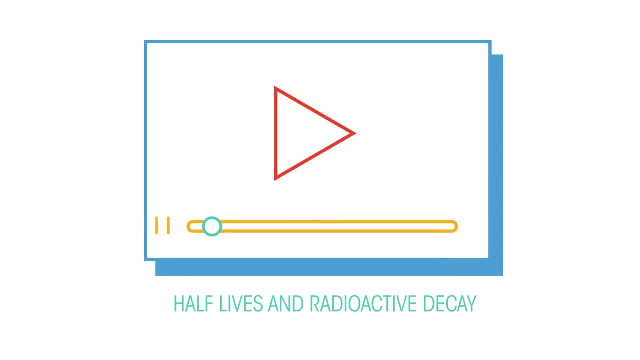 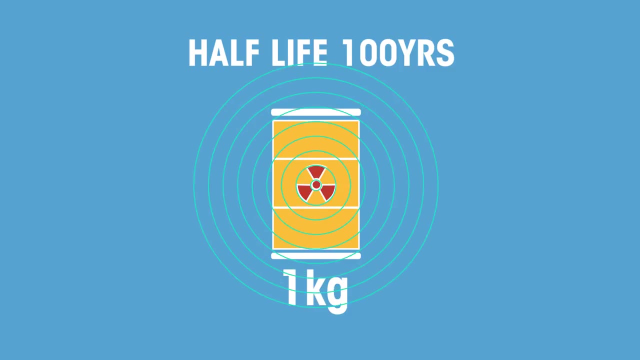 depending upon the different half-lives. Half-lives mean the level of hazard of the radioactive waste reduces with time. To learn more about half-lives, visit our website at wwwradioactivewastecom. If we start off with a kilogram of radioactive waste that has a half-life of 100 years.